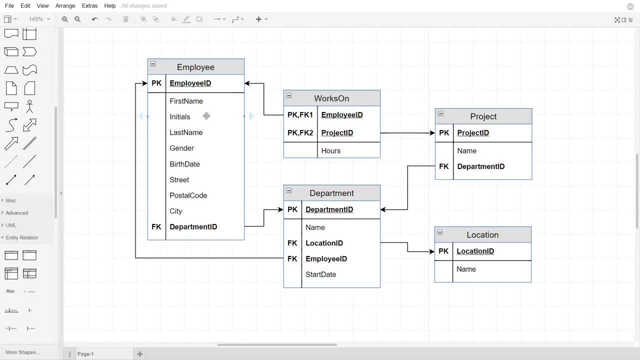 composite attributes when we made this relational data model, but we only chose the simple parts. we also have a primary key here. it's a combined primary key consisting of employee ID and project ID, and then we have the hours. we also have a primary key here. name: we have also a name on the department. we have a location. 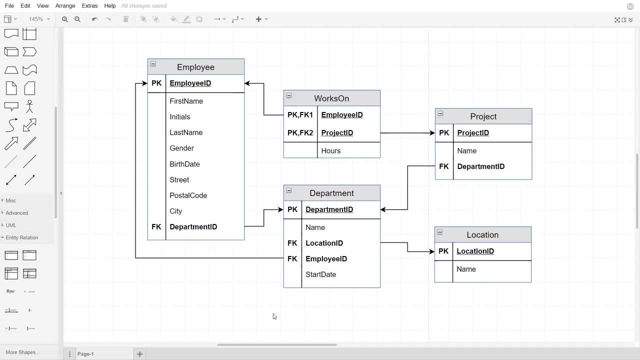 name right here and we don't have any multifur 니mals value attributes. well, actually we did have one on the location for Department, but when we convert the ER diagram into the relational data model, we created a new table so we didn't have the multivalued anymore. so this should satisfy the first. 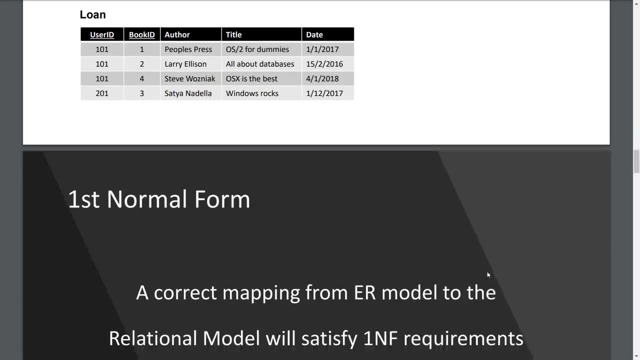 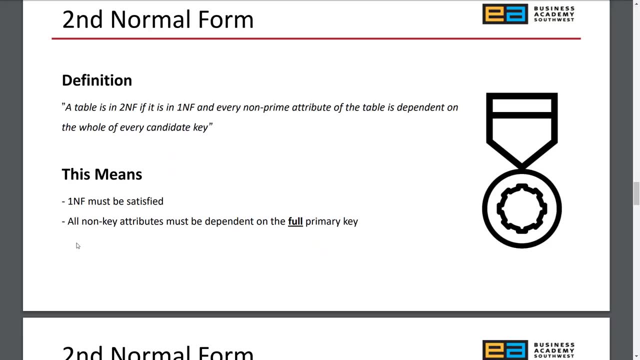 normal phone. if we take a look at the second normal phone, you can see here the table must satisfy the first normal phone and then, furthermore, all non key attributes must be dependent on the full primary key and most often this could be a problem if you have a combined primary. 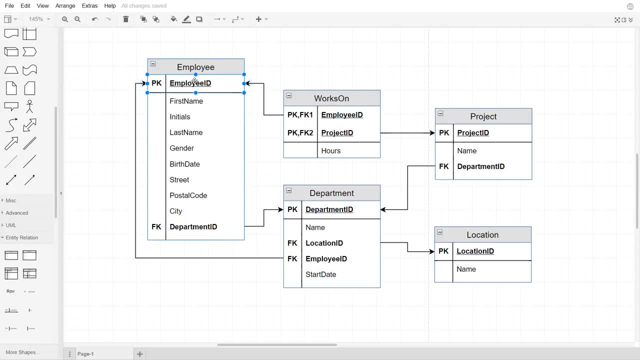 key. we can see here that in the employee table we only have one primary key and they all depend on that. in the work zone, which is actually a many-to-many table, we have a combined primary key, but we can see that this is the working hours that an employee works on a project, so this is also dependent on both of these. 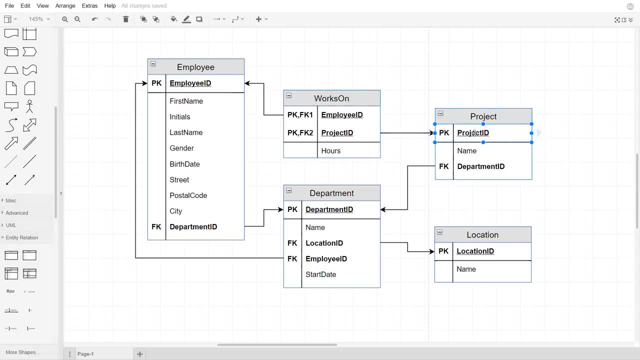 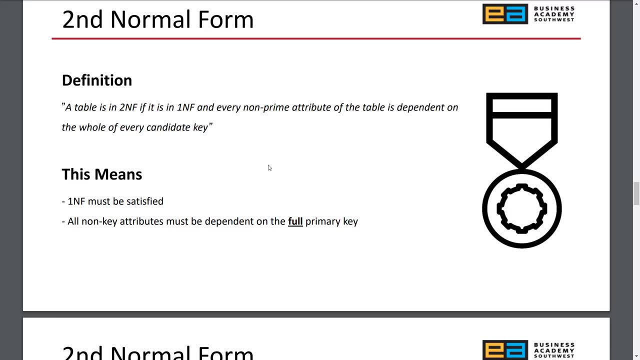 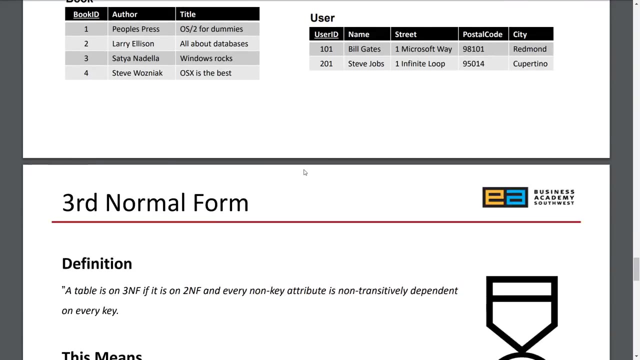 these columns. here we have one primary key, here we have one for the location, one for the department that they're dependent on. so our relational data model should also satisfy the second normal form. and this takes us to the third. one third normal form says that the table should be on the second normal. 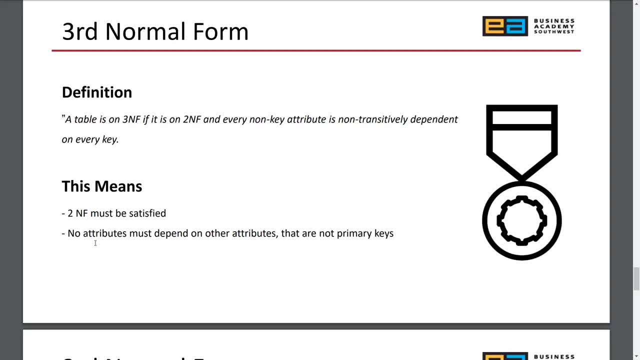 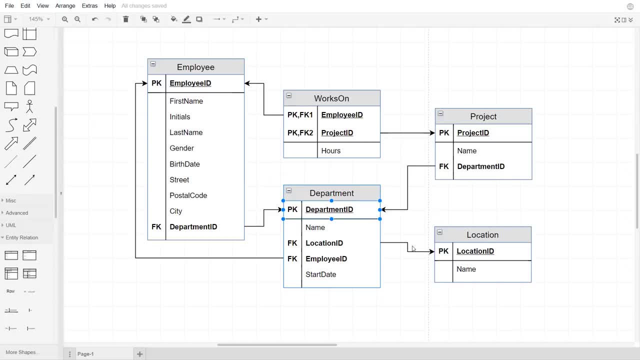 form and furthermore- and that is important- no attributes must depend on other attributes that are not primary keys. and if we take a look here, we can see that this is okay. here, this is okay. we only have one, one attribute. here, this is okay. the department is also. 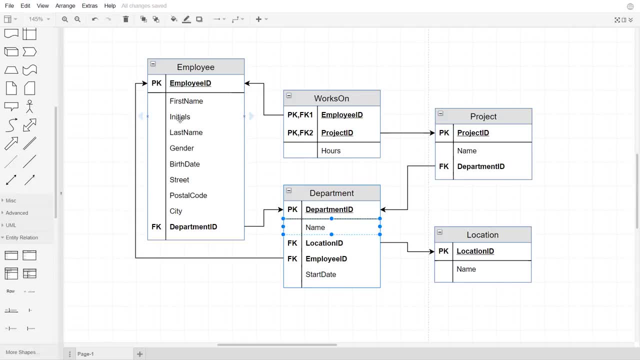 okay. the employee first name, initials, last name, gender, birthday, street is okay. postal code- city. this could be a problem because postal code and city are actually dependent on each other and they are- they're not keys. they are not primary key or foreign keys. if we change the postal code, then the city will change as well. so city depends on postal. 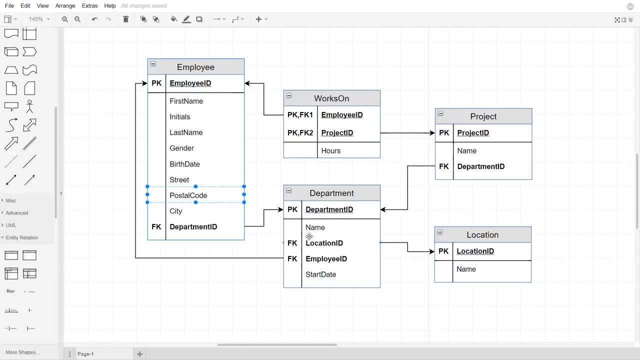 code. so how do we handle that? one way to do that is to create a new table, and here we can call it postal code. here let's see postal code, and then we will put the city. so we have the postal code, we have the city, and then we can remove the city from the employee table. and furthermore, 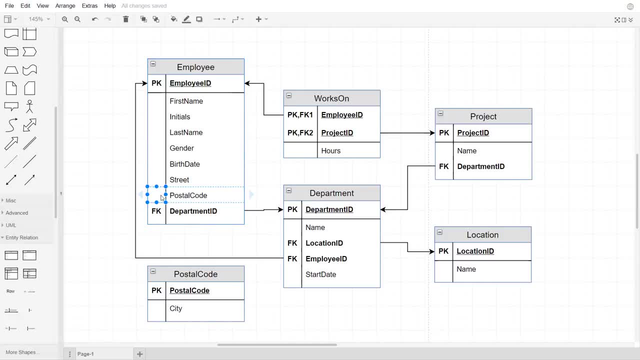 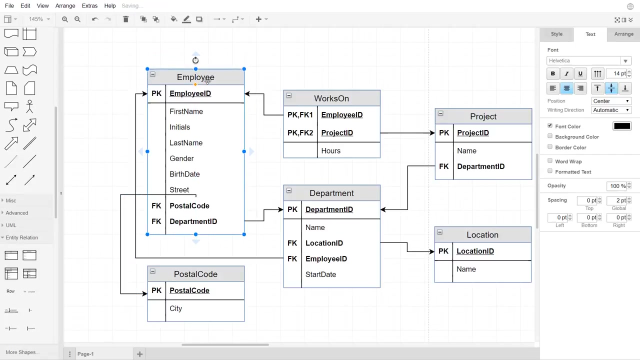 we need to connect these two tables, so we need to make this a foreign key and it should reference the postal code, and we're just going to make this bold here and finally we can make a connection to that. so now we can see here if we can make this correct. 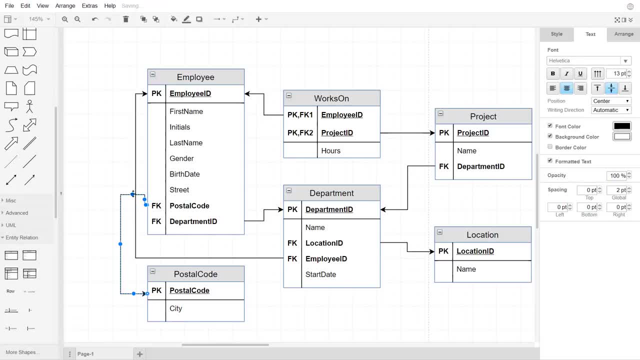 directly. all right, now we have the postal code- that is, a foreign key referencing the postal code table- and then we have the city, and this will prevent us from having duplicate data in the employee table, because we only have one table of the city. all right, this. 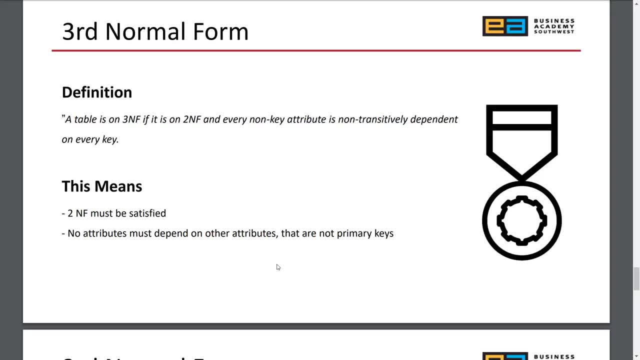 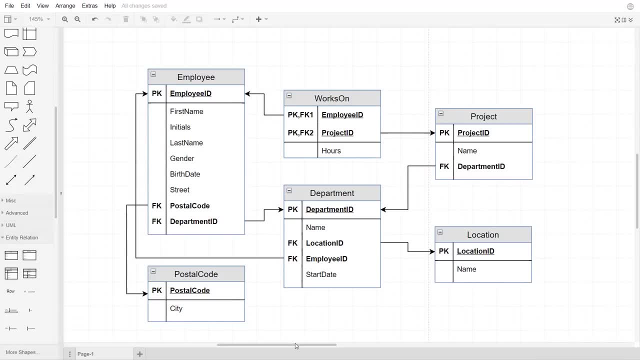 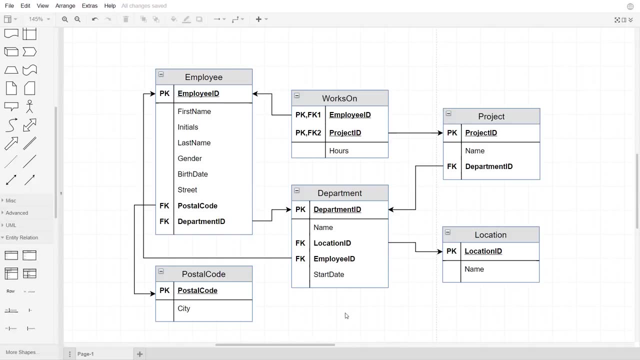 actually concludes our normalization process. we have normalized our table to the third normal form and this will this will ensure that our database is optimized to a certain level. thank you very much for watching. bye, bye.